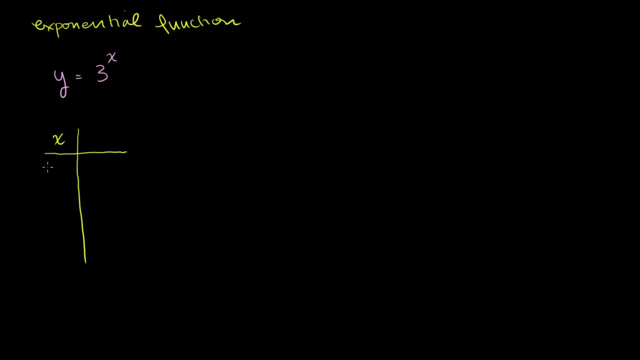 So let's take some x values here. So let's say, let's start with: x is equal to negative 4.. Then we'll go to negative 3, negative 2,, 0,, 1,, 2,, 3, and 4.. 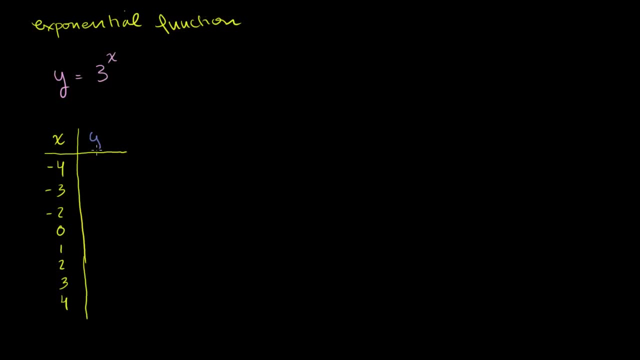 And let's figure out what our y values are going to be for each of these x values. Now here, y is going to be 3 to the negative 4 power, which is equal to 1 over 3 to the fourth power. 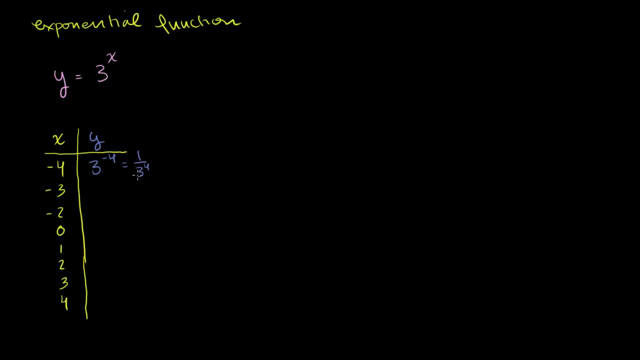 3 to the third is 27,. times 3 again is 81. So this is equal to 1 over 81. When x is equal to negative 3, y is 3.. Let me do this in a different color. 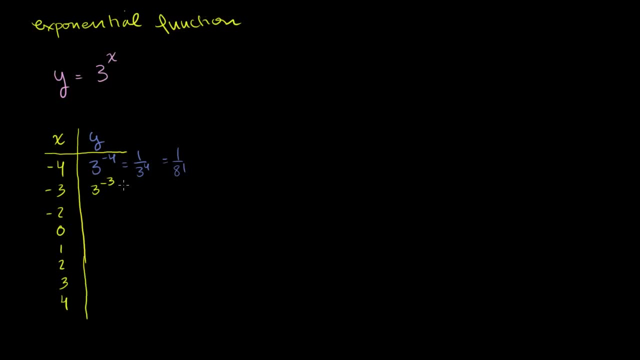 That color's hard to read. y is 3 to the negative 3 power. Well, that's 1 over 3 to the third power, which is equal to 1 over 27.. So we're going from a superposition. 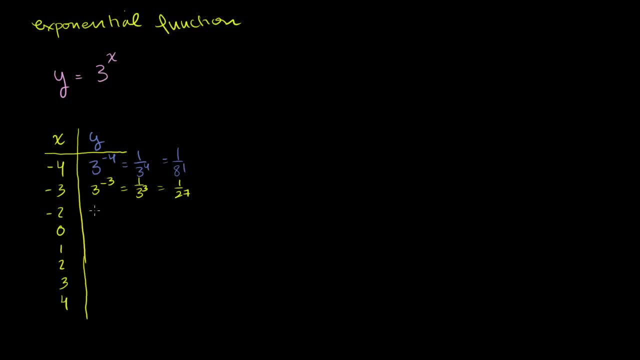 It's a super small number to a less super small number. And then 3 to the negative 2 power is going to be 1 over 9.. 1 over 3 squared, And then we have 3 to the 0 power, which is just equal to 1.. 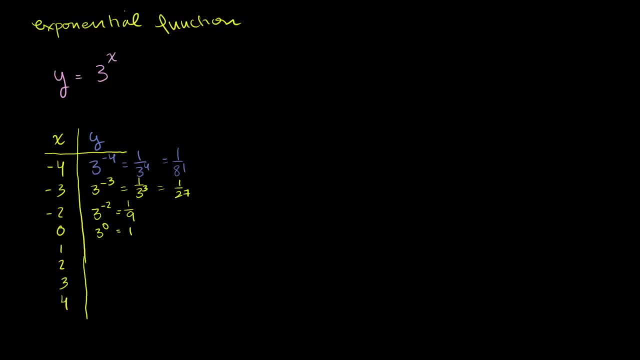 So we're getting a little bit larger, a little bit larger, But we're going to see we're about to explode. Now we have 3 to the first power, That's equal to 3.. Then we have 3 to the second power. 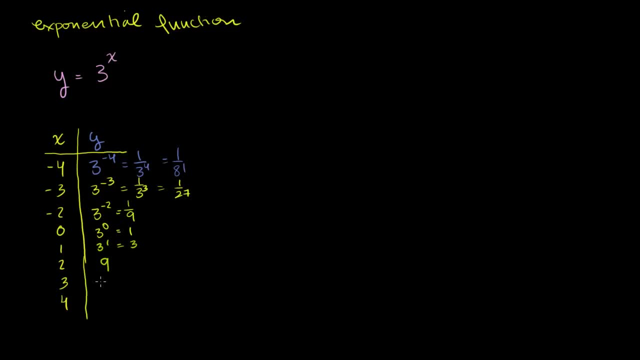 y is equal to 3 to the second power, That's 9.. 3 to the third power: 27.. 3 to the fourth power: 81.. If we were to put the fifth power, 243.. Let's graph this just to get an idea of how. 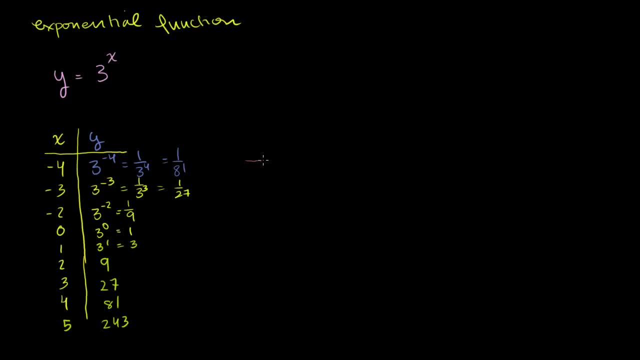 quickly, we're exploding. So let me draw my axes here. So that's my x-axis And that is my y-axis. That is my y-axis, And let me just do it in increments of 5, because I really want to get the general. 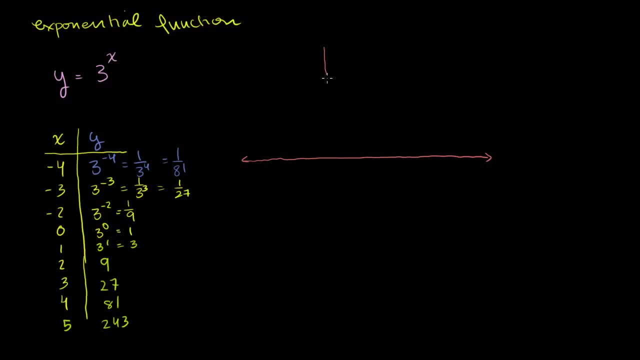 general shape of the graph here. So let me just draw as straight a line as I can. Let's say this is 5,, 10,, 15.. Actually I won't get to 81 that way. I want to get to 81.. 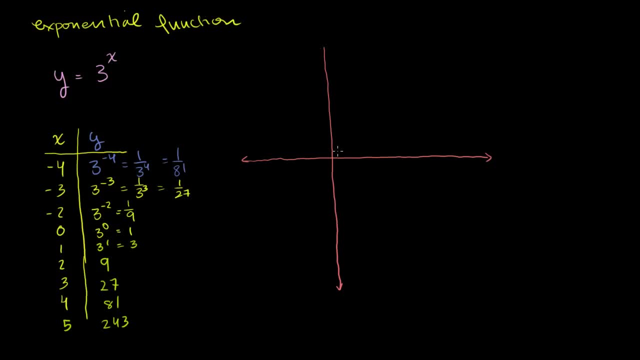 Actually, well, that's good enough. Let me draw it a little bit differently than I've drawn it. So let me draw it down here, Because all of these values you might notice are positive values, because I have a positive base. 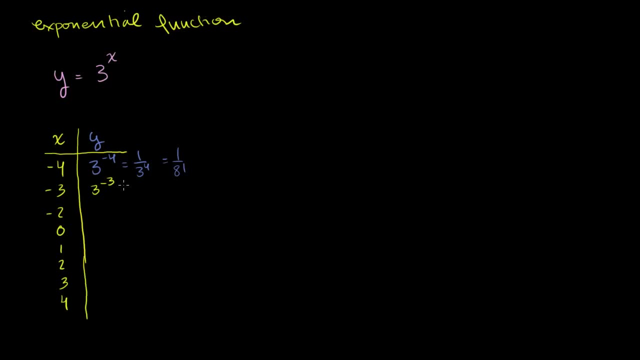 That color's hard to read. y is 3 to the negative 3 power. Well, that's 1 over 3 to the third power, which is equal to 1 over 27.. So we're going from a super-power to a negative power. 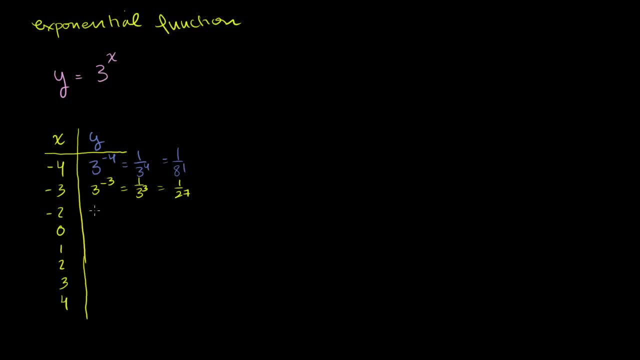 From a super-small number to a less super-small number, And then 3 to the negative 2 power is going to be 1 over 9.. 1 over 3 squared, And then we have 3 to the 0 power, which is just equal to 1.. 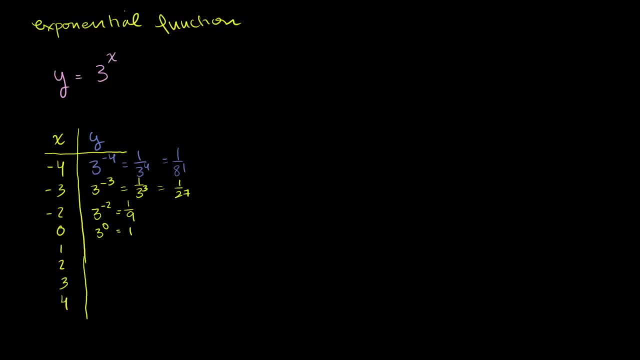 So we're getting a little bit larger, a little bit larger, But we're going to see we're about to explode. Now we have 3 to the first power, That's equal to 3.. Then we have 3 to the second power. 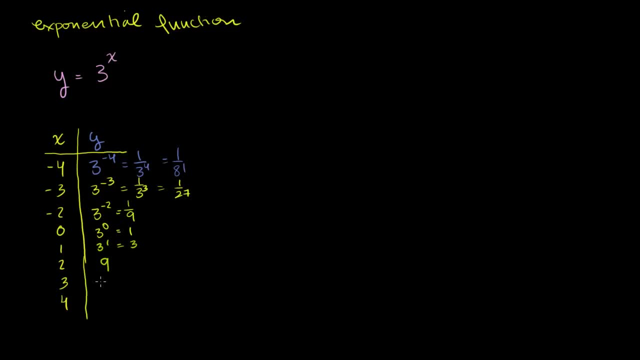 y is equal to 3 to the second power, That's 9.. 3 to the third power: 27.. 3 to the fourth power: 81.. If we were to put the fifth power, 243.. Let's graph this just to get an idea of how. 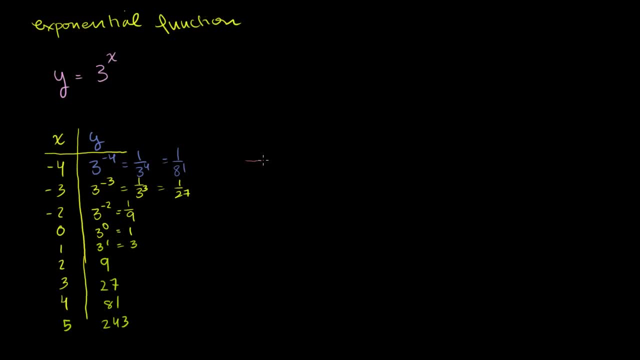 quickly we're exploding. So let me draw my axes here. So that's my x-axis and that is my y-axis, And let me just do it in increments of 5, because I really want to get the generalization, I want to get the general shape of the graph here. 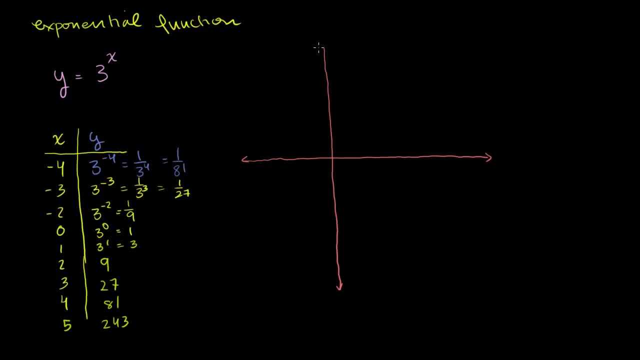 So let me just draw as straight a line as I can. Let's say this is 5,, 10,, 15.. Actually, I won't get to 81 that way. I want to get to 81. Actually, well, that's good enough. 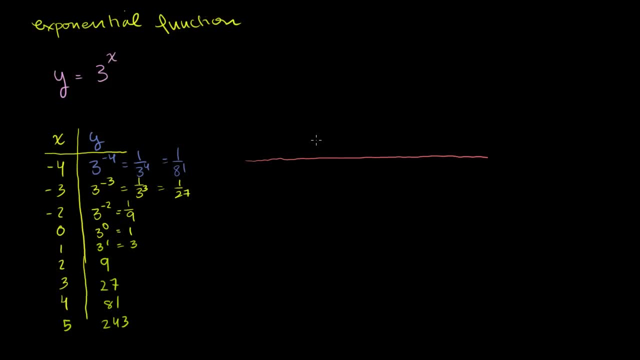 Let me draw it a little bit differently than I've drawn it. So let me draw it down here, Because all of these values, you might notice, are positive values, because I have a positive base, So let me draw it. Let me draw it like this, like that. 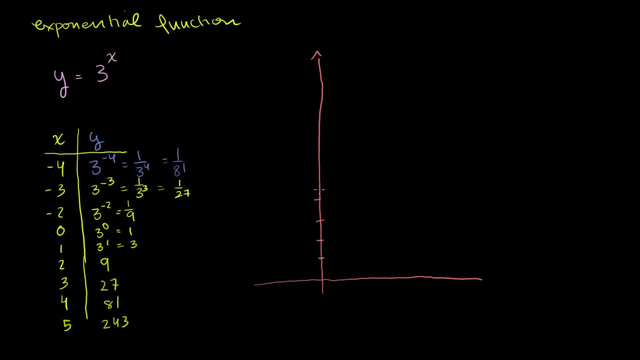 Good enough. And then let's say: I have 10,, 20,, 30,, 40,, 50,, 60,, 70,, 80.. That is 80, right there. That's 10.. That's 30.. 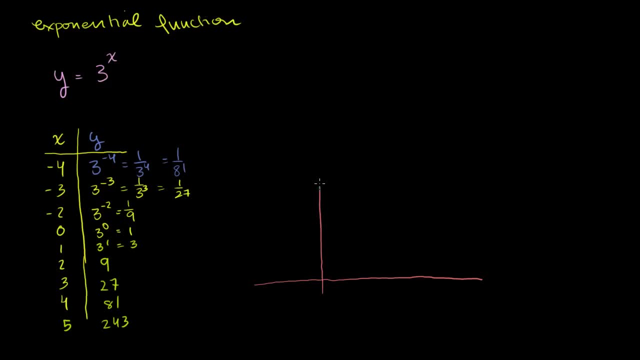 So let me draw it. Let me draw it like this, Like that, Good enough. And then let's say, I have 10, 20,, 30,, 40,, 50,, 60,, 70,, 80.. That is 80, right there. 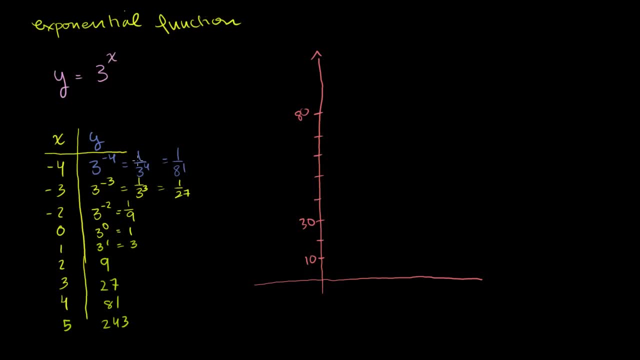 That's 10.. That's 30.. That'll be good for approximation. And then let's say that this is negative 5.. This is positive 5, right here. And actually let me stretch it out a little bit more- Say this is negative 1.. 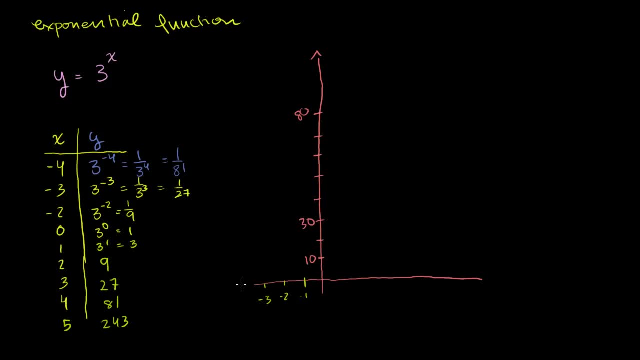 Negative, 2. Negative, 3. Negative, 4.. And then we have 1,, 2,, 3, and 4.. So, when x is equal to 0,, we're equal to 1,, right. When x is equal to 0,, y is equal to 1,, which is maybe right around there. 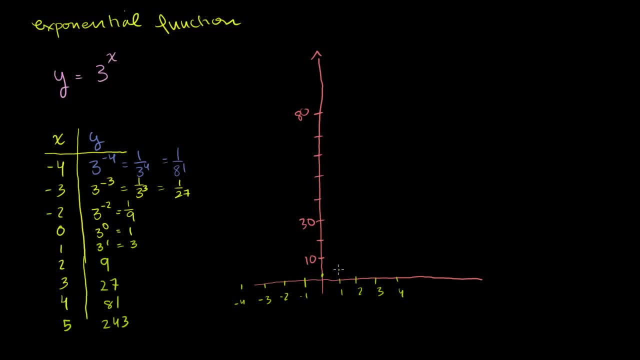 When x is equal to 1, y is equal to 3, which is maybe right around there. When x is equal to 2, y is equal to 9,, which is right around there. When x is equal to 3, y is equal to 12.. 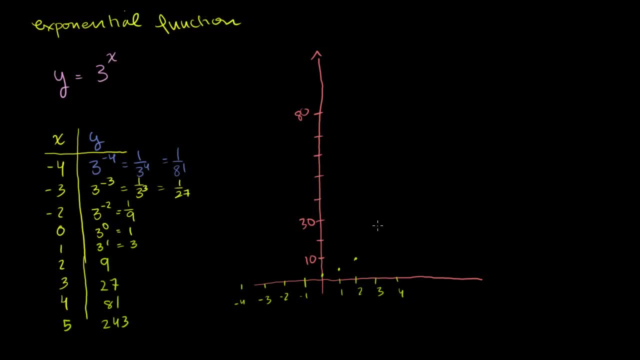 y is equal to 27,, which is right around there. When x is equal to 4,, y is equal to 81.. y is equal to 81.. So you see very quickly, this is just exploding. If I did 5, we'd go to 243, which wouldn't even fit on my screen. 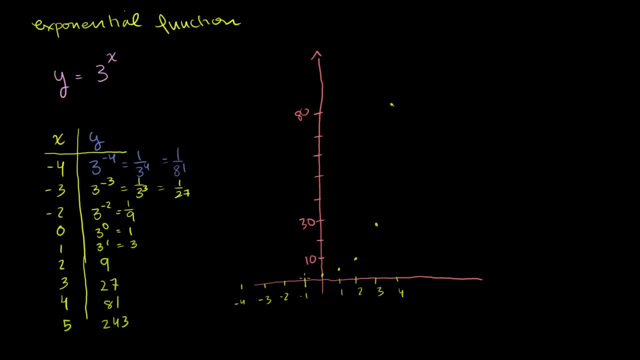 When you go to negative 1, we get smaller and smaller. So at negative 1, we're at 1, 9th, I mean eventually, you're not even going to see this. It's going to get closer and closer to 0.. 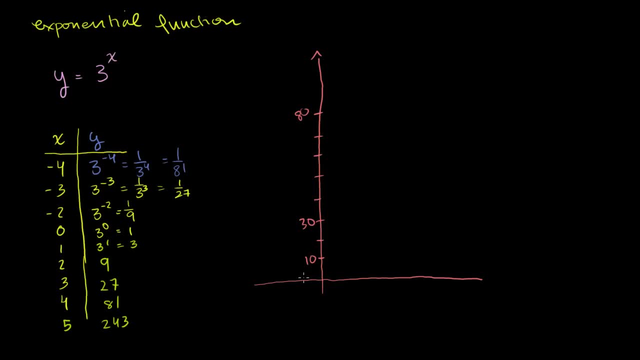 That'll be good for approximation. And then let's say that this is negative 5.. This is positive 5, right here. And actually let me stretch it out a little bit more- Say this is negative 1.. Negative 2, negative 3, negative 4.. 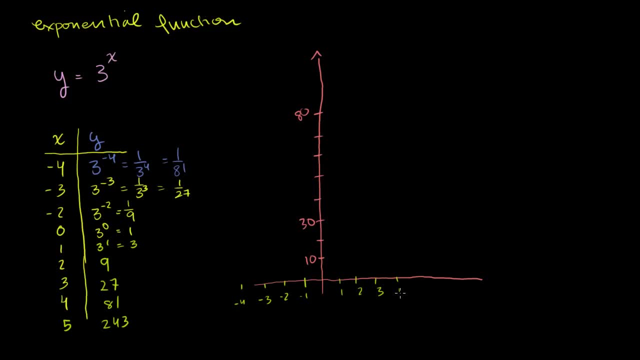 And then we have 1,, 2,, 3, and 4.. So when x is equal to 0, we're equal to 1, right? When x is equal to 0, y is equal to 1, which is maybe. 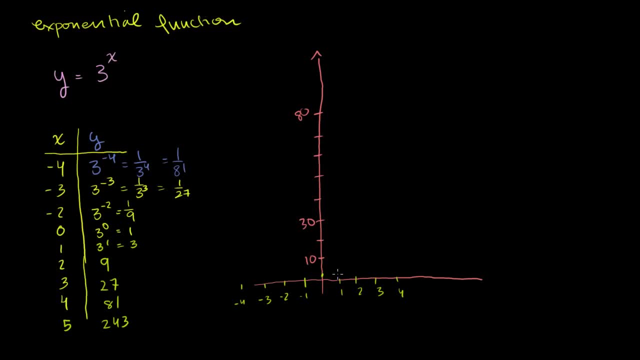 right around there. When x is equal to 1, y is equal to 3,, which is maybe right around there. When x is equal to 2, y is equal to 9,, which is right around there. When x is equal to 3, y is equal to 20.. 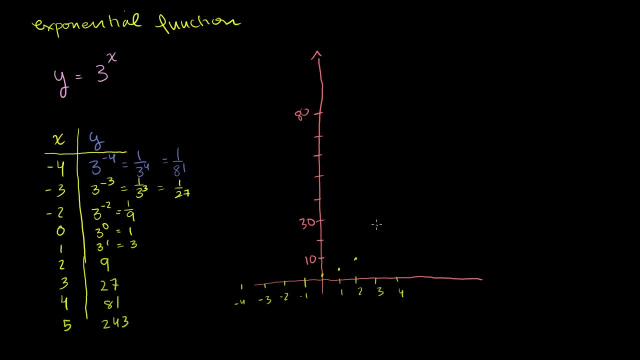 27, which is right around there. When x is equal to 4, y is equal to 81.. So you see very quickly this is just exploding. If I did 5, it would go to 243,, which wouldn't even. 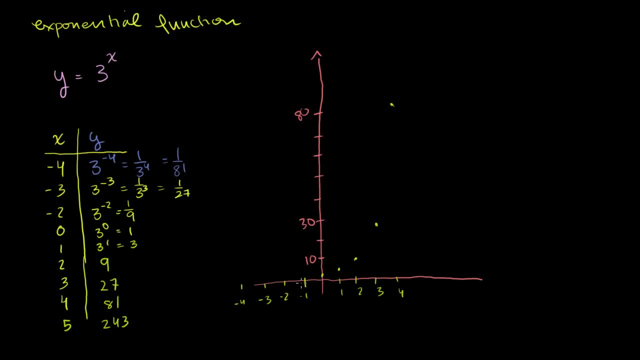 fit on my screen. When you go to negative 1, we get smaller and smaller. So at negative 1, we're at 1 ninth. I mean eventually, you're not even going to see this. It's going to get closer and closer to 0.. 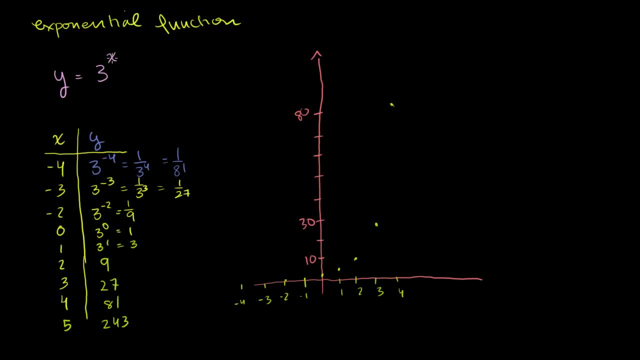 As this approaches larger and larger negative numbers, or I guess I should say smaller negative numbers. so 3 to the negative 1,000, 3 to the negative 1,000,000,. we're getting numbers closer and closer to 0. 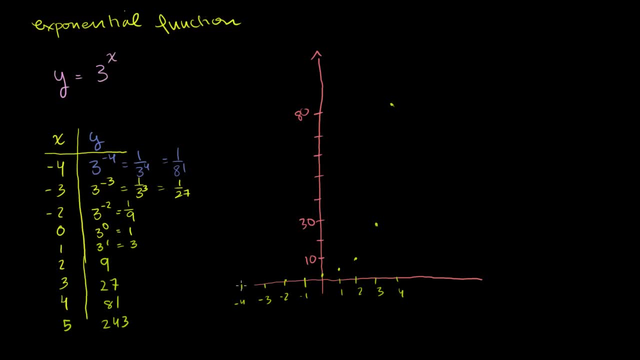 without actually ever approaching 0. So as we go from negative infinity- x is equal to negative infinity- we're getting very close to 0. We're slowly getting ourselves away from 0. But then bam, once we start getting to the positive numbers, we just explode. 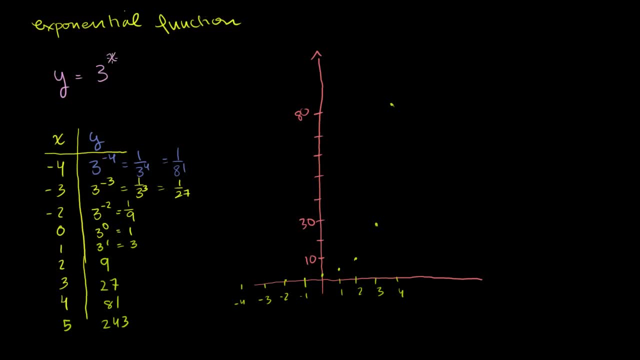 As this approaches, larger and larger negative numbers, or I guess I should say smaller numbers, Negative numbers. So 3 to the negative 1,000, 3 to the negative 1,000,000.. We're getting numbers closer and closer to 0. 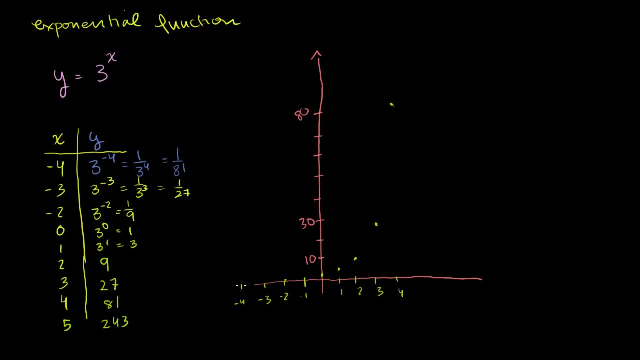 without actually ever approaching 0. So as we go from negative infinity- x is equal to negative infinity- we're getting very close to 0. We're slowly getting ourselves away from 0. But then bam, once we start getting into the positive. 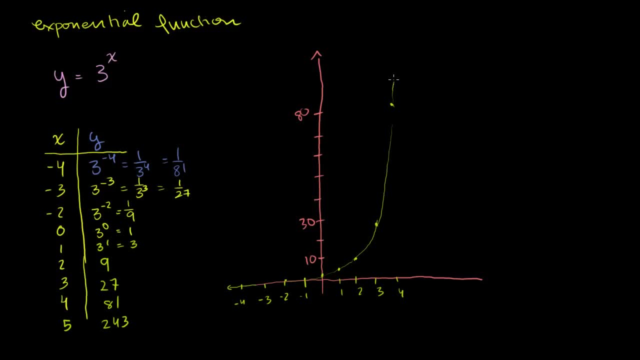 numbers. we just explode, We just explode and we keep exploding at an ever-increasing rate. So the idea here is just to show you that exponential functions are really, really dramatic. Well, you can always construct a faster expanding function. For example, you could say: y is equal to x to the x. 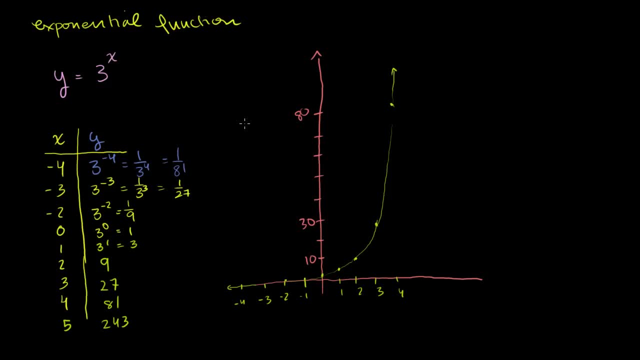 even faster expanding. But out of the ones that we deal with in everyday lives, this is one of the fastest. So, given that, let's do some word problems that just give us an appreciation for exponential functions. So let's say that someone sends out a chain letter on. 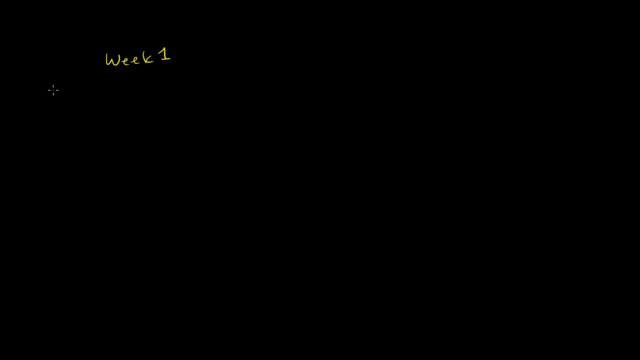 let's say in week 1.. So in week 1, someone sends a chain letter to 10 people And the chain letter says: you have to now send this chain letter to 10 more new people And if you don't, you're going to have bad luck. 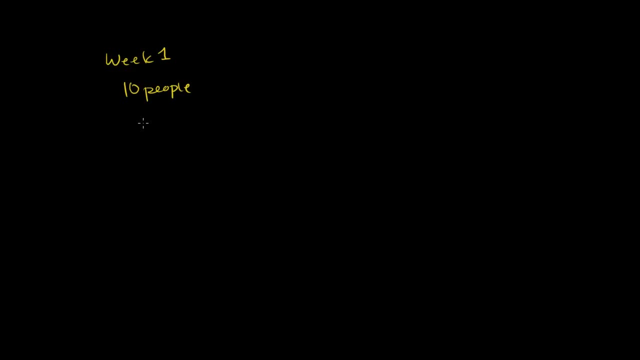 and your hair's going to fall out and you'll marry a frog or whatever else. So all of these people agree and they go and each send it to 10 people the next week. So in week 2, they go out and each send it. 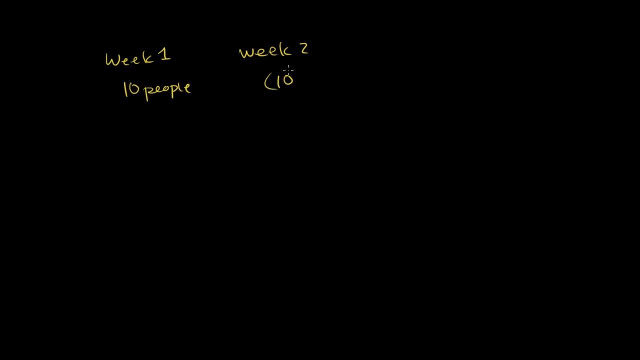 to 10 more people. So each of those original 10 people are each sending out 10 more of the letters. So now 100 people have the letters right. Each of those 10 sent out 10.. So that 100 letters were sent out. 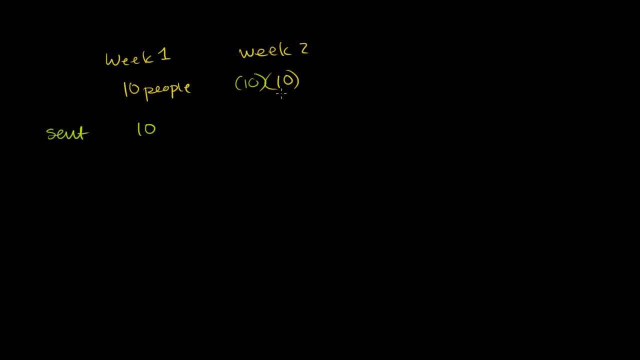 So let me see Sent. 10 were sent Here, 100 were sent In week 3, what's going to happen? Each of those 100 people who got this one, they are each going to send out 10,. 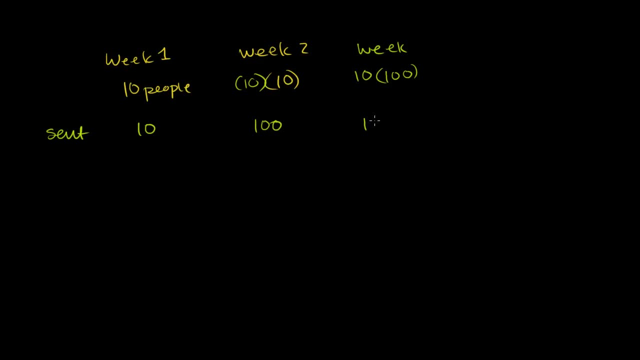 assuming that everyone is really into chain letters. So a 1,000.00.. A 1,000.00 people are going to get them, And so the general pattern here is the people who receive it. So in week n, where n is the week we're talking about? 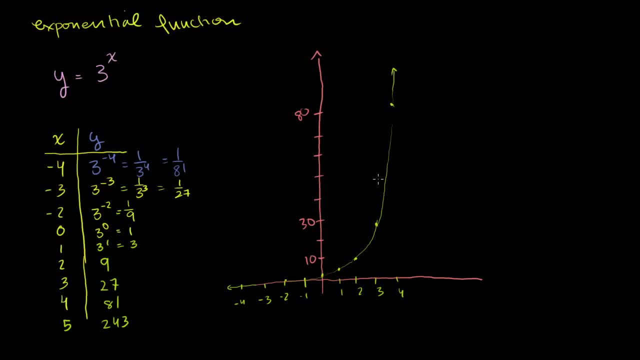 We just explode and we keep exploding at an ever-increasing rate. So the idea here is just to show you that exponential functions are really, really dramatic, That they're the kind of well you can always construct a faster expanding function. 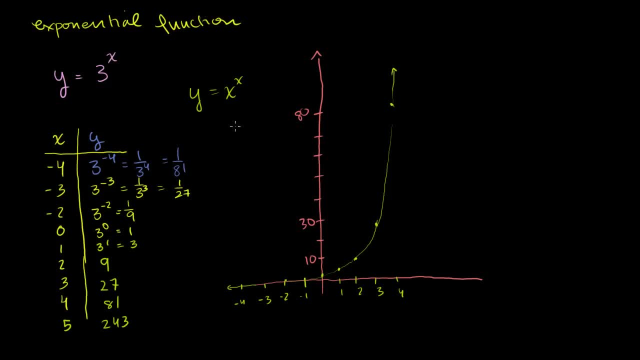 For example, you could say: y is equal to x, to the x even faster expanding. But out of the ones that we deal with in everyday lives, this is one of the fastest. So, given that, let's do some word problems that just give us an appreciation. 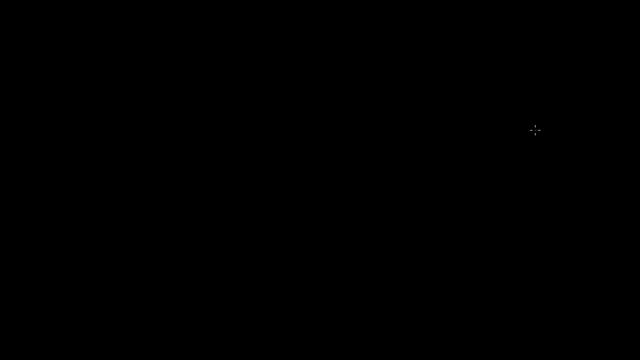 for exponential functions. So let's say that someone sends out a chain letter on, let's say, in week 1.. Week 1. Someone sends a chain letter to 10 people And the chain letter says: you have to now send this chain letter to 10 more new people. 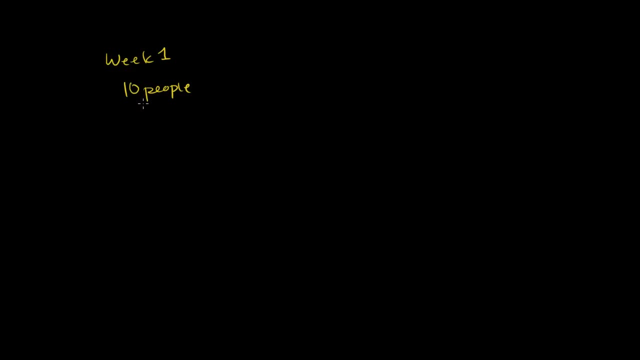 And if you don't, you're going to have bad luck and your hair's going to fall out and you'll marry a frog or whatever else. So all of these people agree and they go and each send it to 10 people the next week. 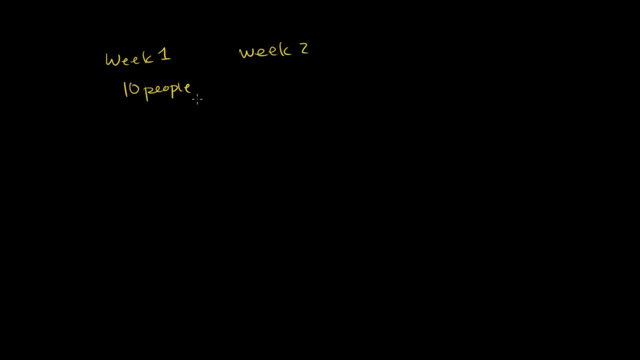 So in week 2, they go out and each send it to 10 more people. So each of those original 10 people are each sending out 10 more of the letters. So now 100 people have the letters right. Each of those 10 sent out 10.. 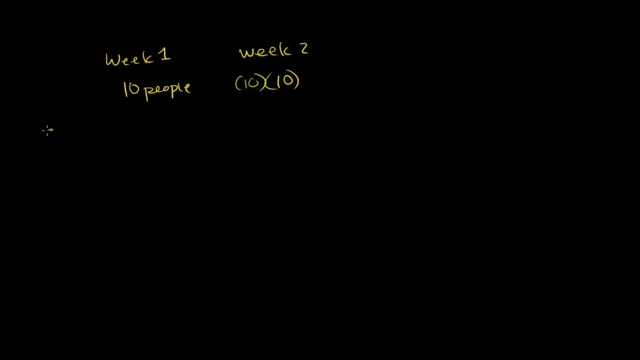 So 100 letters were sent out. So let me see Sent: 10 were sent Here, 100 were sent In week 3, what's going to happen? Each of those 100 people who got this one, they're each going to send out 10,. 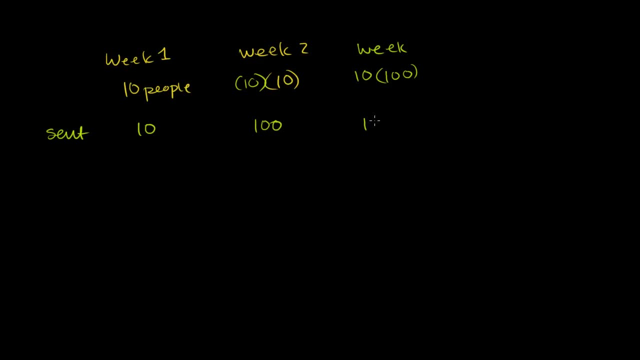 assuming that everyone is really into chain letters. So 1,000 people are going to get them, And so the general pattern here is the people who receive it. So in week n, where n is the week, we're talking about how many people receive the letter. 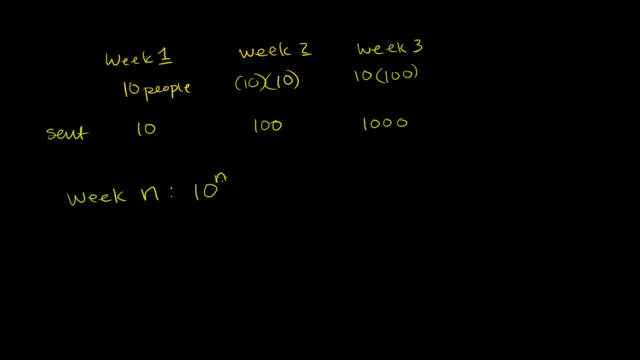 In week n we have 10 to the nth. people receive i before e except after c, The letter. So if I were to ask you how many people are getting the letter on the sixth week, how many people are actually going to receive that letter? 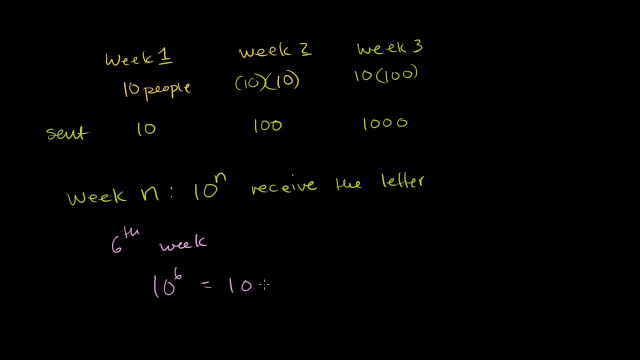 Well, what's 10 to the sixth power? 10 to the sixth is equal to 1, with six zeros, which is 1 million people are going to receive that letter in just six weeks, just sending out 10 letters each, And obviously in the real world. 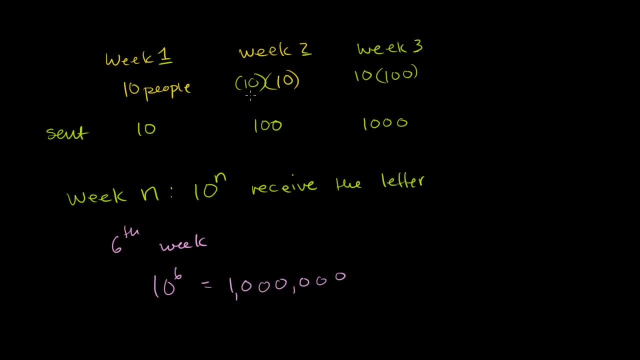 most people chuck these in the basket. so you don't have this good of a hit rate. But if you did, if every 10 people you sent it to also sent it to 10 people, and so on and so forth, by the sixth week you would have a million people.